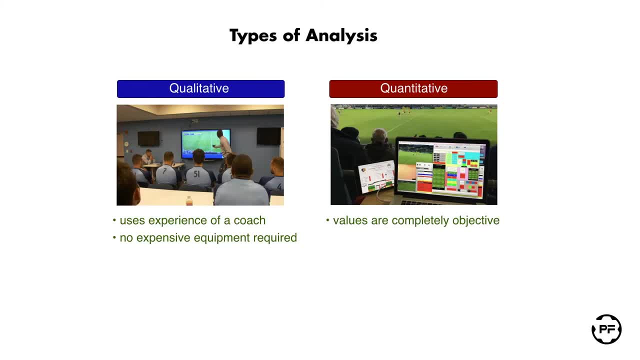 Qualitative analysis doesn't require expensive equipment and can be conducted very easily, Whereas quantitative data can be accessed anytime and used for comparison between current and previous performances. The problem of qualitative analysis is that research demonstrated that coaches have limited recall ability and do not remember all the events that occurred during the game. 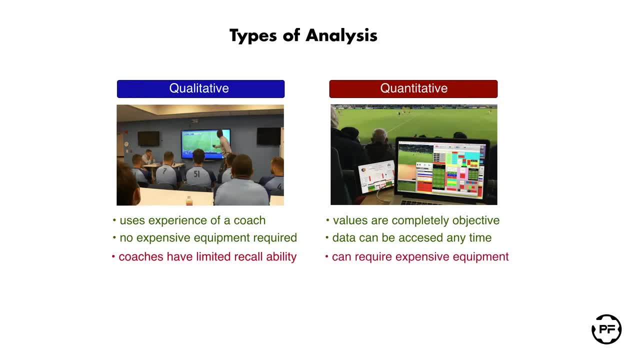 At the same time, quantitative analysis usually requires expensive equipment and not all football clubs can afford it. Research also demonstrated that coaches are open to personal bias, emotions and high levels of subjectivity, whereas quantitative data can be easily taken out of context and misinterpreted when judged. 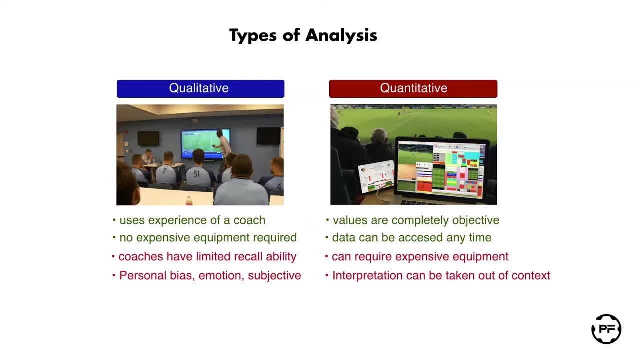 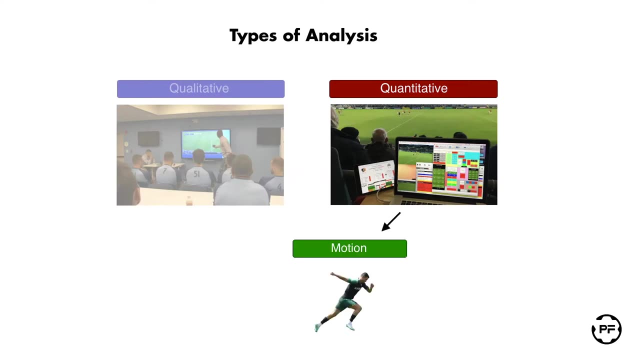 by inexperienced coaches or analysts. To be a successful football coach, you will need to combine both of these methods. Because qualitative analysis is pretty obvious, we are going to consider just the quantitative one. Quantitative analysis is further divided into motion and notational analysis. 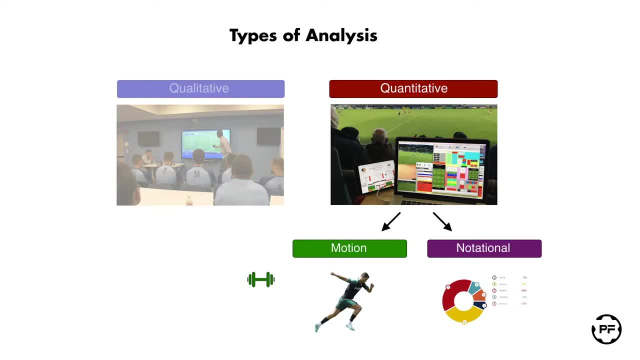 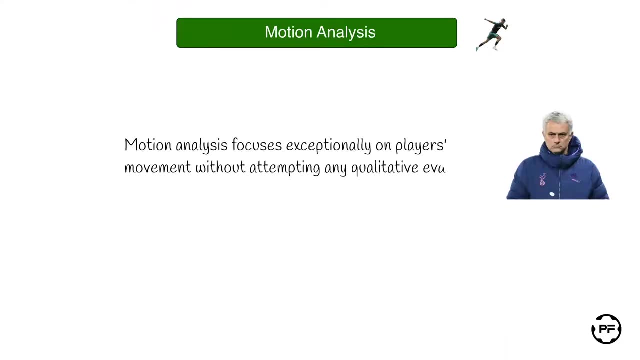 Motion analysis focuses exceptionally on the physical aspect of performance, whereas notational considers technical, tactical and psychological aspects. Let's first start with motion analysis. Motion analysis focuses exceptionally on player's movement without attempting any qualitative evaluation. Some examples include total distance covered, the overall amount of sprints performed and 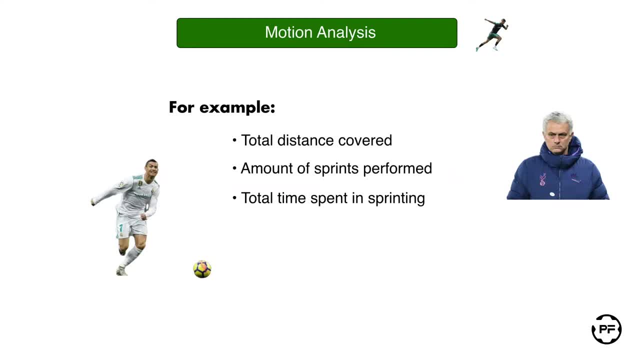 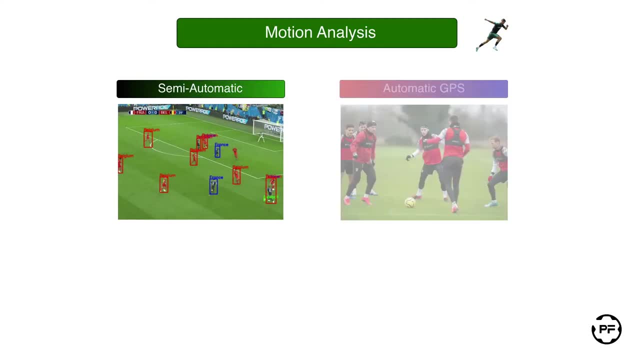 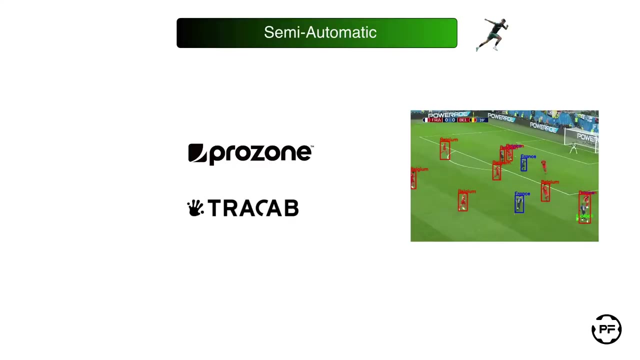 total time spent in sprinting. Motion analysis can be either semi-automatic or an automatic GPS analysis. Let's first start with the semi-automatic analysis. The most known providers of semi-automatic solutions are Prozon and TriCarp. These systems rely on cameras that need to be installed at a home stadium to track every 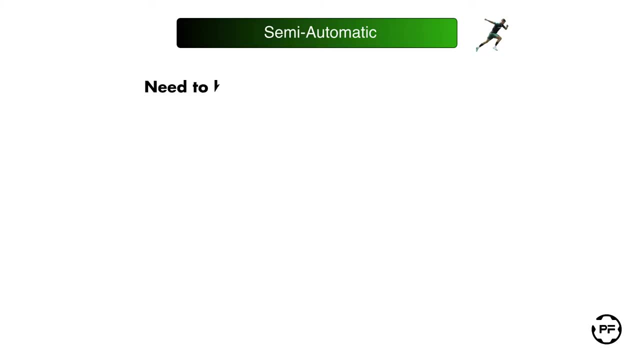 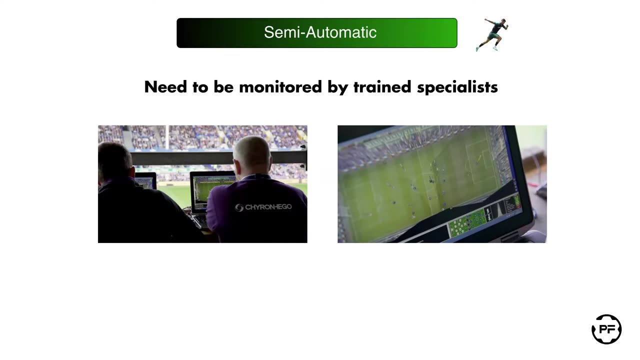 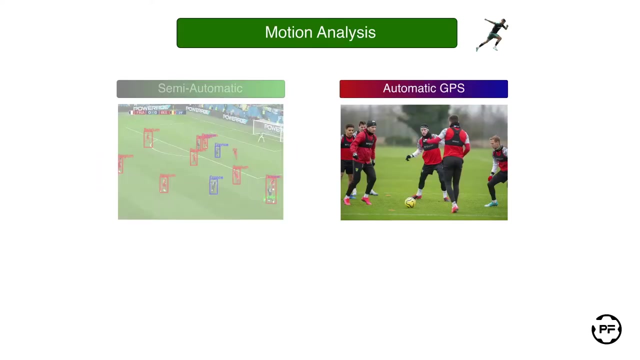 player on the pitch. Semi-automatic solutions need to be monitored by specialists, who correct tracking errors when players are bench-tapped in restricted playing areas. That's why such systems are just semi-automatic. OK, let's now have a look at fully automatic GPS systems. 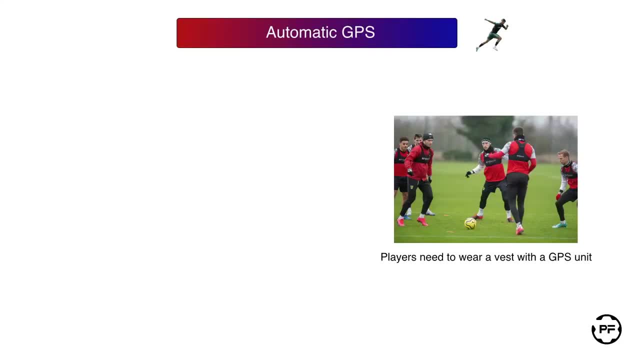 These systems require players to wear a relatively inobtrusive vest that contains a GPS unit. The most known providers are Catapult, GPSports and Statsports Having the same functionality as semi-automatic systems. GPS systems additionally provide information on training intensity and performance. 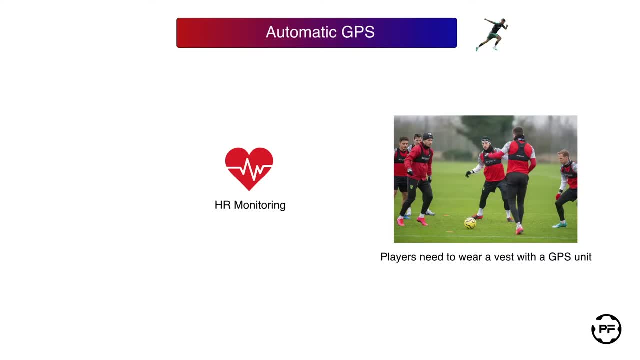 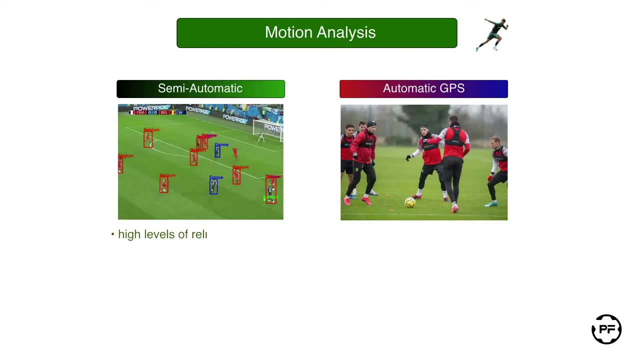 These systems can be used to track players' physical activity via monitoring players' heart rates. OK, let's now compare semi-automatic and automatic GPS systems one by one. The advantages of semi-automatic systems are that they have very high levels of reliability and validity and there is no need for players to wear any transmitting devices. 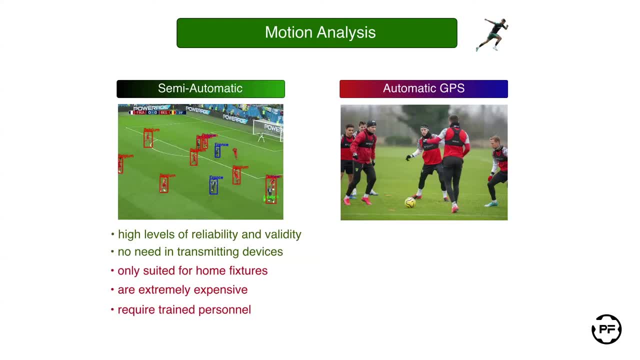 Because cameras need to be installed at a home stadium. semi-automatic systems are only suited for home fixtures, personal to ensure their correct functioning. In contrast, in GPS systems, the data is gathered completely automatically, with no need for any intervention. They are also portable and relatively inexpensive, so can equally be used during away matches. 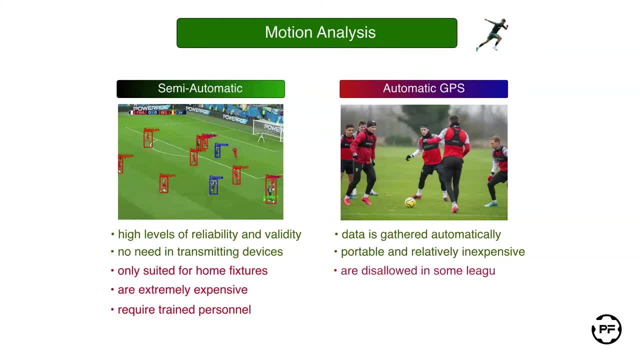 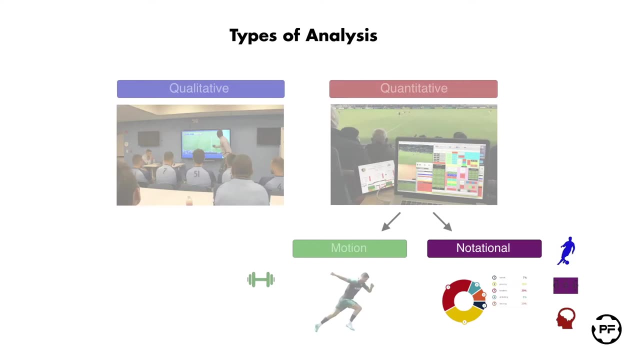 and sessions. Unfortunately, GPS systems are still disallowed in some leagues and competitions. Also, some players might feel uncomfortable knowing they are constantly monitored. OK, let's finally consider the notational systems. Notational analysis represents an objective way of recording performance, so that critical 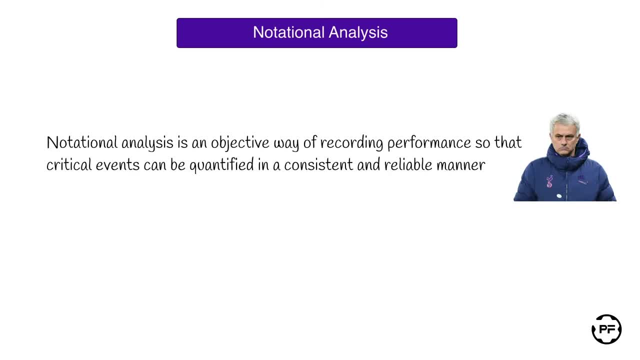 events can be quantified in a consistent and reliable manner. Most notational systems record the following parameters: The action performed, together with the outcomes, The player that performed that action, The time of the action and the position where the action took place, According to your needs. 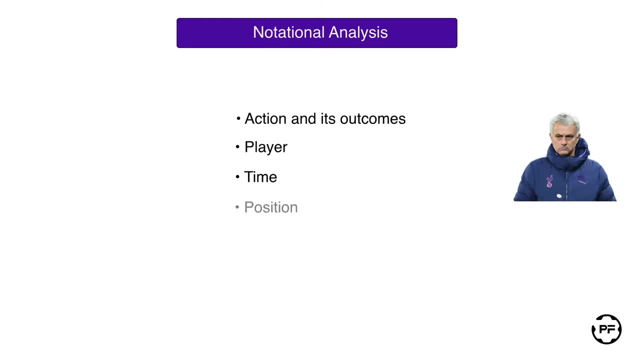 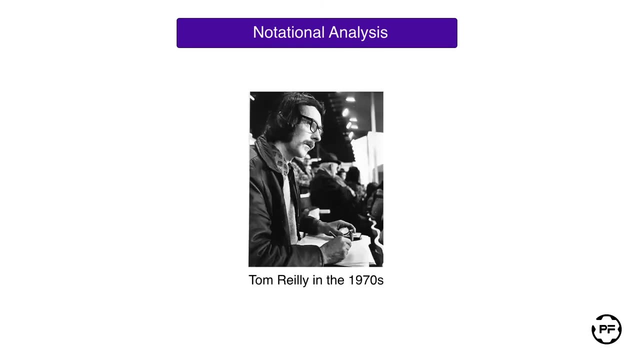 You can record just some of them, For example, just action, player and time, Or only action and its position. The father of notational analysis was professor Thomas Riley, who worked closely with Everton Football Club and first used the pen and paper approach to quantify match performance. 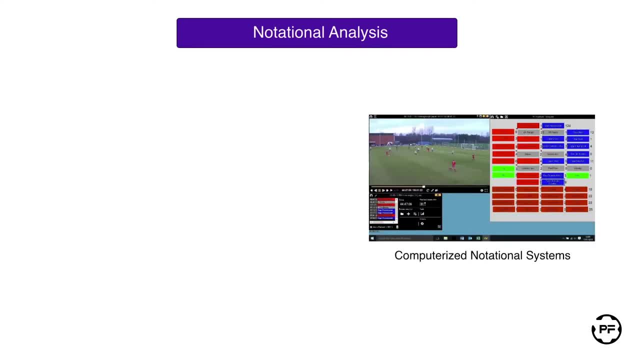 But today's performance analysts make use of computerized notational systems. The most known providers are Nuxpot, Dartfish and Spotscode. Let's have a closer look at Nuxpot, the favorite notational system of Unai Emery. 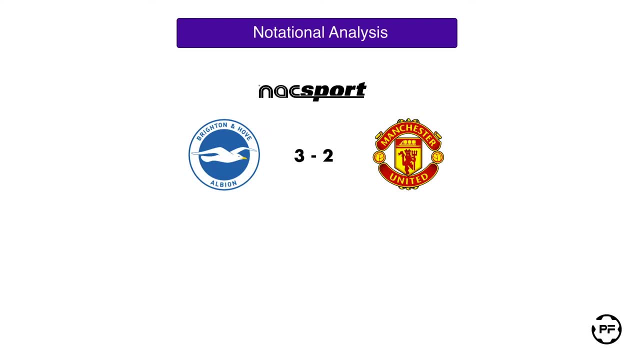 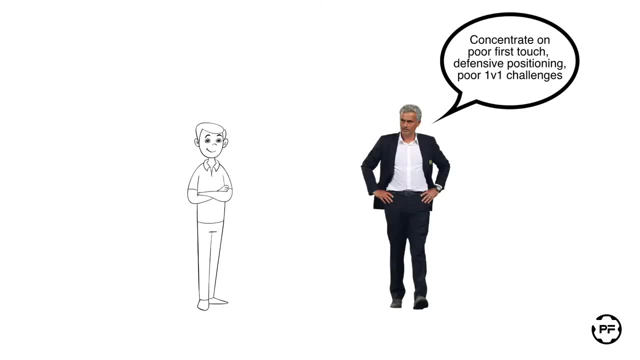 In Nuxpot you are going to analyze the defeat of Manchester United against Brighton as part of the 18-19 Premier League season, And the head coach asks you to pay attention to poor first touches, defensive positioning and poor one-on-one challenges. 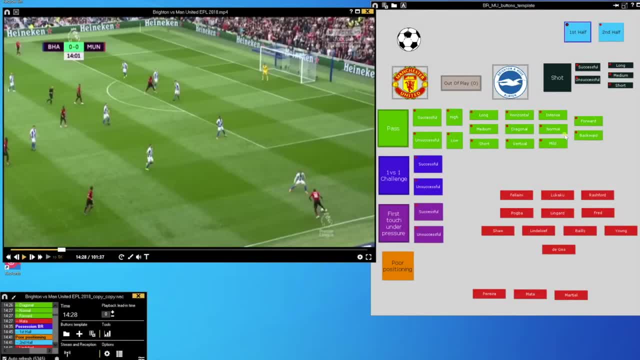 OK, let's look at the right first. Here you can see our specially designed buttons template. Let's take a look at the right first. Here you can see our specially designed buttons template. And because Jose was interested in poor one-on-one challenges, poor first touch under pressure. 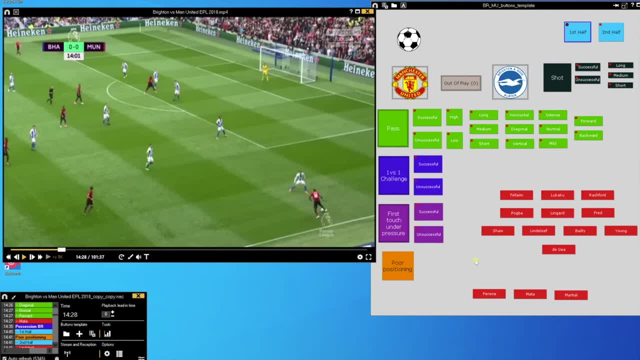 and poor positioning. we added exactly these buttons to the template. For example, when you see a one-on-one challenge at the video on the left, you can click on the one-on-one challenge button. You specify whether it was successful or unsuccessful and which player performed that challenge. 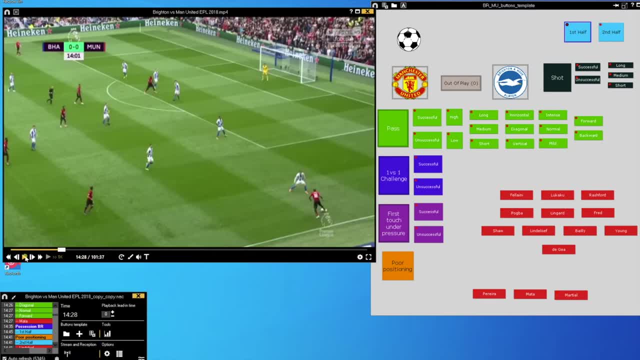 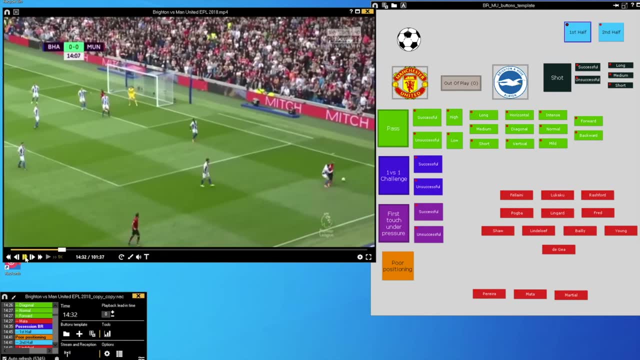 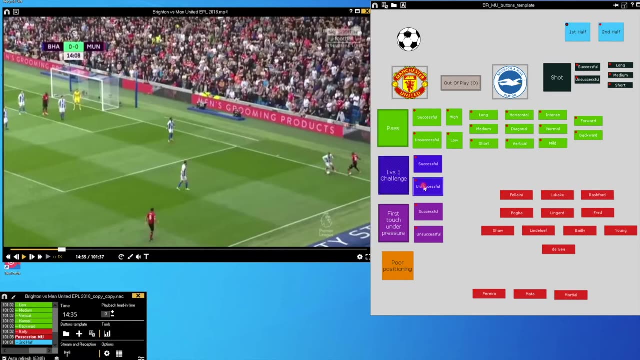 Let's now have a look at an example. Here you can see a poor one-on-one challenge performed by Ashley Young, So you can stop the playback, click one-on-one challenge button. unsuccessful and Ashley Young. And from now it is stored inside our database. 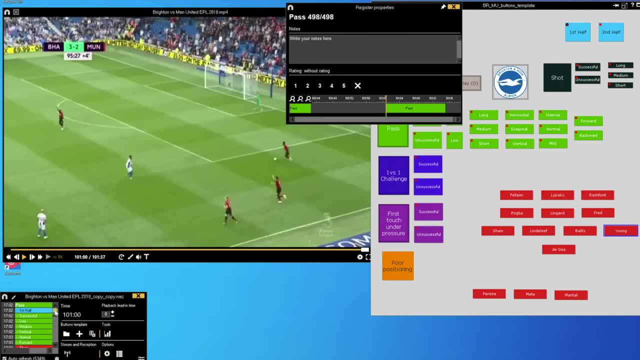 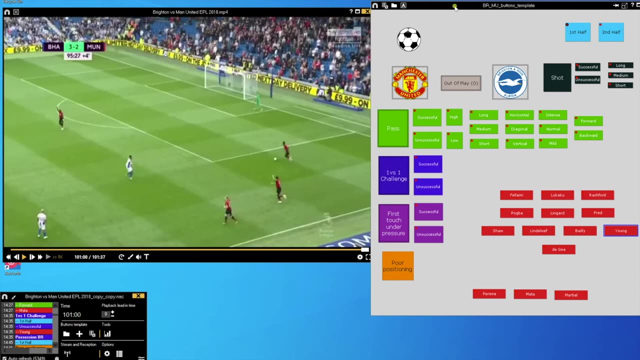 Let's check it on the left panel. Yeah, here you see, one-on-one challenge. first house that has been added automatically: unsuccessful: Young. In this way, we keep on gathering all the stats of the actions that Jose was interested in. Once we have all the required data collected, we can go to our dashboard and take a look. 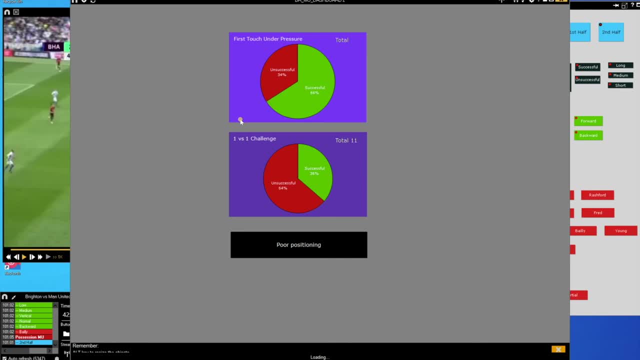 at some charts Here you see that one-third of first touches under pressure and two-thirds of one-on-one challenges have been unsuccessful. This is a pretty big number so we can report it later to Jose. And if you click on unsuccessful first touches you can see all the situations where Manchester 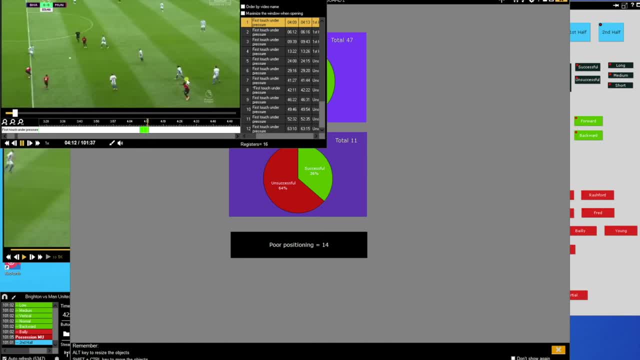 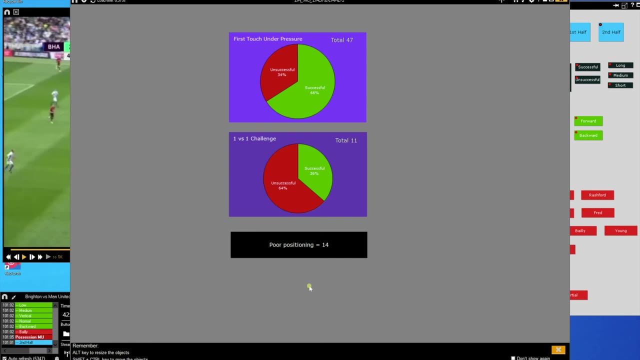 players performed a poor first touch Here. you just saw the one by Lukaku. You can then easily export all these videos into one file and present it to the head coach. The same with poor positioning. You can see that throughout the game we've got 14 critical positioning issues. 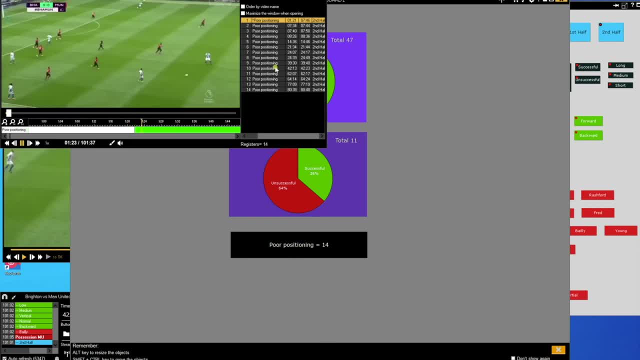 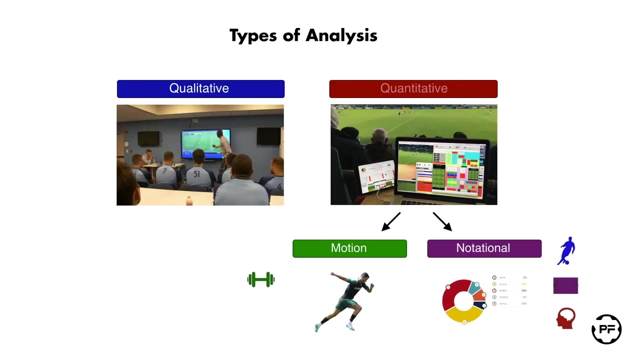 And again, if you click on the label, you can see all of them and present it later to Jose. In this particular case, you might notice the very large distance between two center backs when protecting the middle. We're not going to consider all knackspot features, but I think you've got an idea of